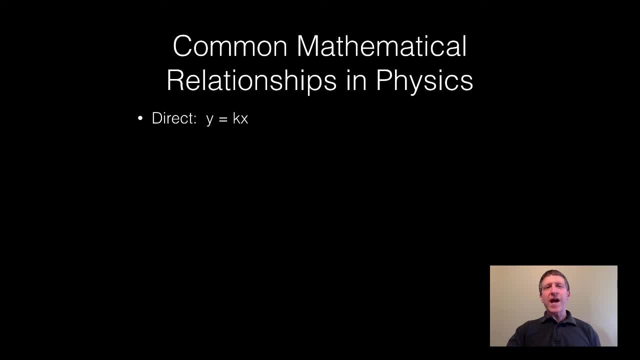 It can appear as a constant in many different types of relationships, not only just linear relationships. This is why I prefer to use k in this regard. So a direct relationship you can express as: y equals y equals k times x. Two variables, y and x, one constant k. 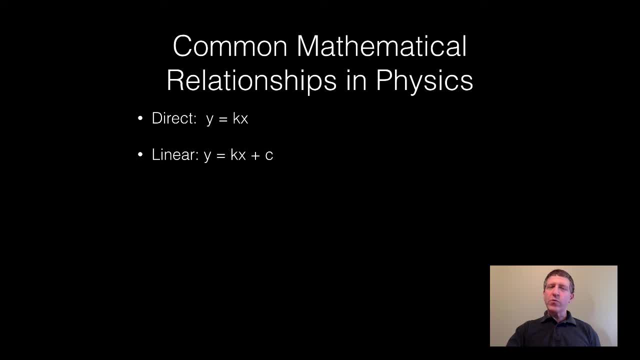 You can also have a linear relationship, which is very closely related to a direct relationship. However, we also have a constant value, sometimes termed a starting point or a vertical intercept c, So this type of graph does not go through the origin. 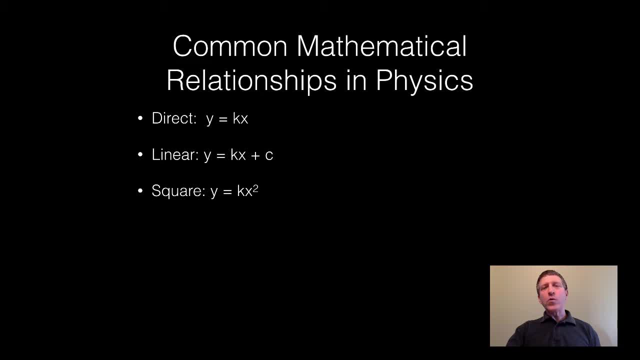 We can have a square relationship where y equals mx and y equals mx. We can have a square relationship where y equals mx and y equals mx. We can have a square relationship where y equals kx squared- some constant k times- x squared. 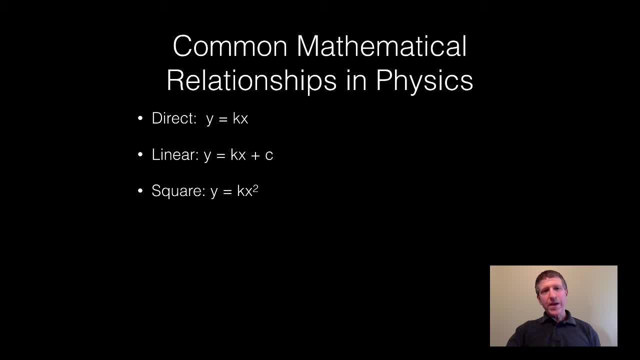 And here's a case where k will not be the slope, so that's why I'm using the letter k there. It is just some constant. We also have a square root relationship. y can equal some constant k times the square root of x. 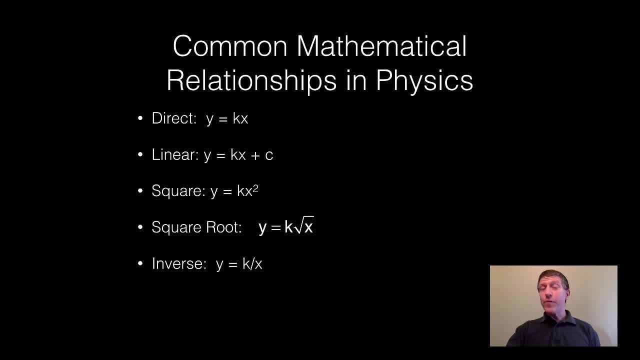 Also an inverse relationship: y equals k over x. Again, k, not the slope in this case. And finally, we could have an inverse square relationship. Again, we could have an inverse square relationship: y equals k over x squared. I'll also briefly mention exponential relationships in this video. 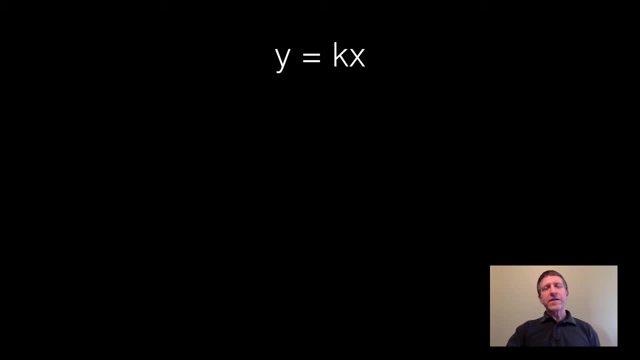 So first we have: y equals k times x. Our variable y, which is typically the dependent variable, equals some constant k times our independent variable x. So another way of writing this is simply: y is proportional to x. If you double x, that means y will double. 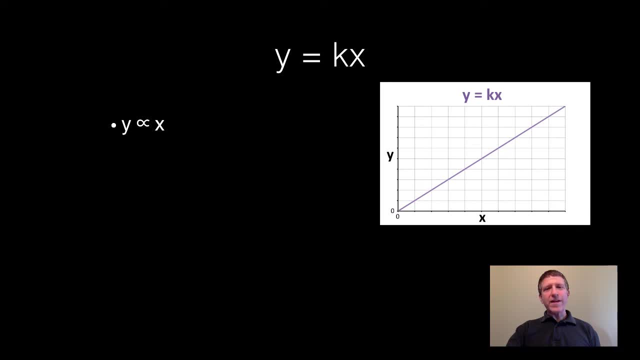 Here's a graph of y equals kx. You can see it's a straight line and it goes through the origin 0, 0.. The way you say this is: y is proportional to x. Or you might say y is directly related to x. 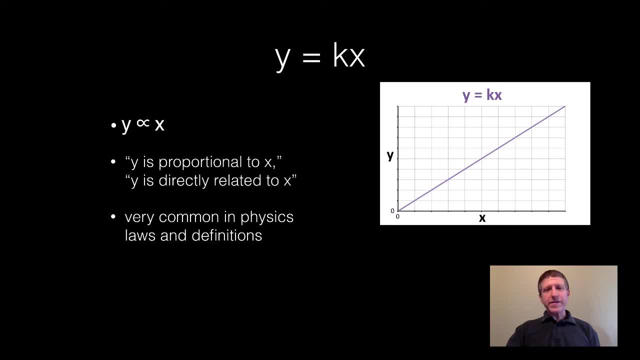 This is a very, very common relationship in physics, in both laws and definitions. Here are some examples where you might see a direct relationship. And even e equals mc squared is a direct proportion. In this case you may say: well, what about that c squared? 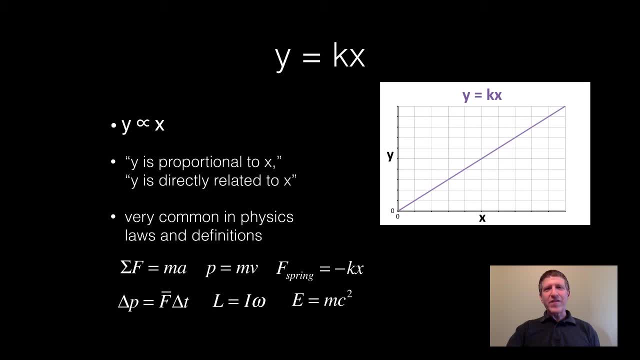 Well, c squared is just a constant. In fact, it may be the most constant thing in the universe. No matter what frame you're in, c is the same thing. So this just shows that e is directly proportional to, or directly related to, the mass of the object. 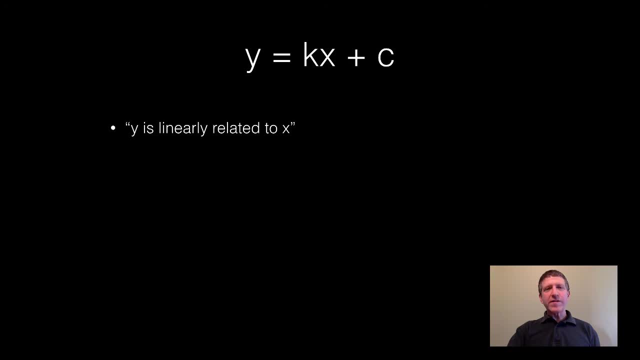 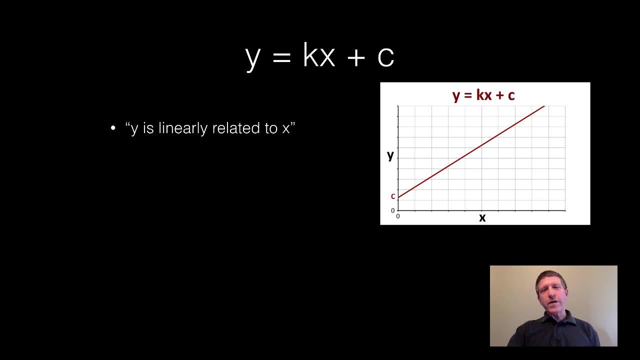 Another common relationship is: y equals kx plus c, Also phrased as y being linearly related to x. And here's a graph of such a relationship. Notice that it is linear, It's a straight line. but it also does not pass through the 0, 0 or the origin. 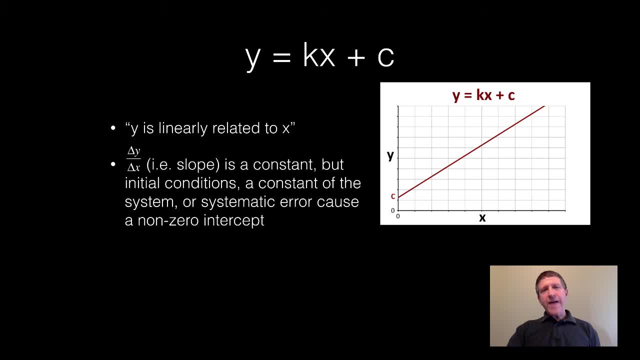 It's got some non-zero vertical intercept And in this type of relationship we do have a constant slope. In other words, delta y over delta x is a constant, But there may be some initial conditions. There may be a constant of the physical system. 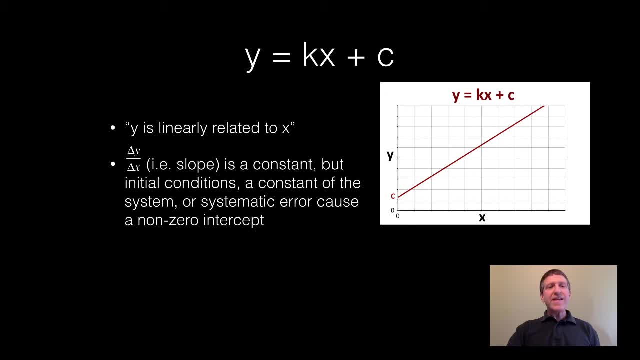 Or there may be even some systematic error which causes a non-zero intercept. A couple of examples. A couple of examples would be: if you graph v versus t, v initial would be the value of v at time equals 0.. If you're exerting a force on a mass but there is kinetic friction, 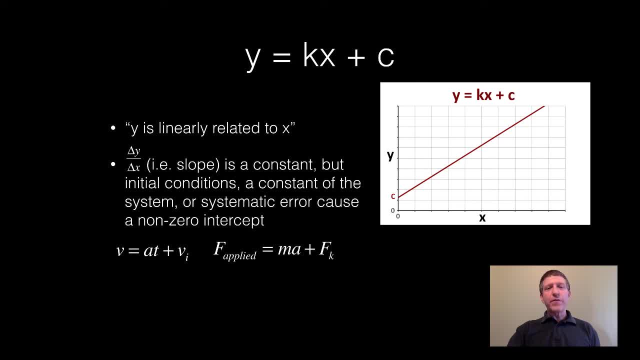 your f sub k would be the vertical intercept. if you graphed the force applied versus the acceleration, That's a constant of the physical system that will show up on our linear graph. You could also have a situation where there's some kind of systematic error. 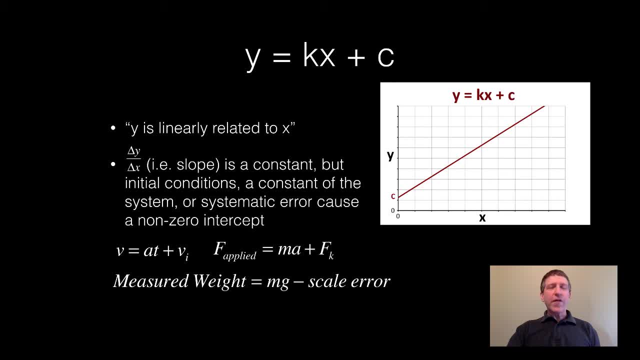 Let's say you're weighing a bunch of masses. Maybe the scale with nothing's on it, is already reading 2 Newtons. We could just graph the measured weight versus the mass of the object And we would get a graph that had slope of g and an intercept of that negative scale error. 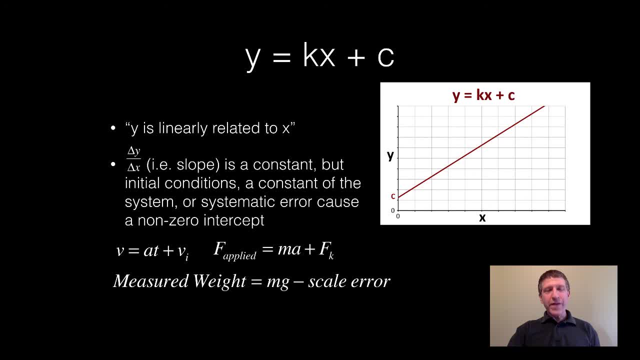 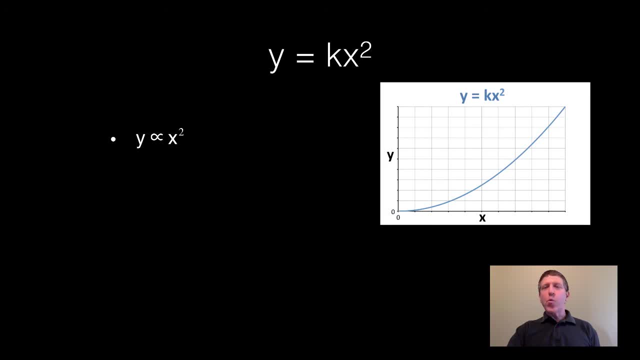 We don't even have to know about it ahead of time. Our graph will reveal that Another common relationship is y equals kx squared. You could say: y is proportional to x squared. This is what that graph looks like And that's the way you'd say it. 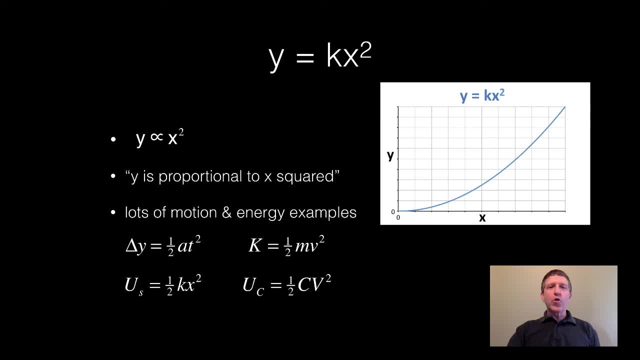 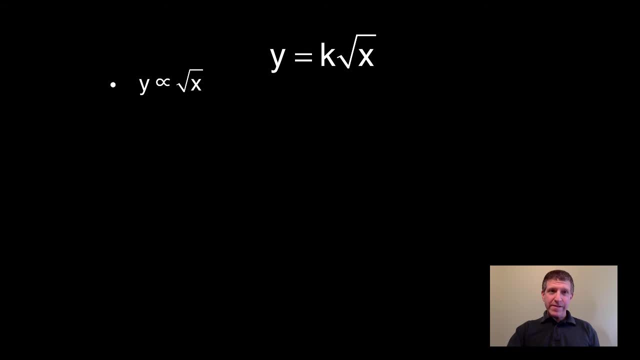 There are a lot of examples of this kind of relationship. Here's a few for motion and energy. Yet another common relationship: y equals k times the square root of x. When you see this, you could say y is proportional to the square root of x. 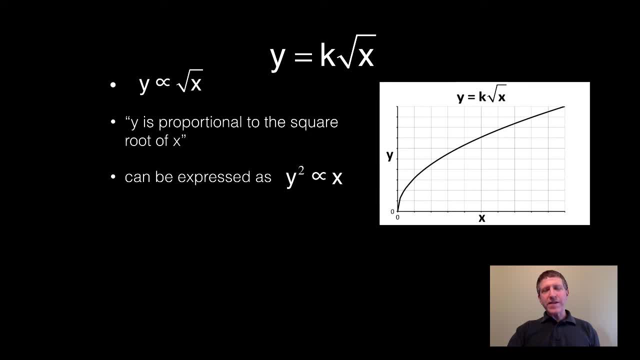 You should note, though, very importantly, you can express this as a square relationship. Notice, if I square both sides of what I have above, you get y squared. Squared is proportional to x. y equals k times the square root of x. 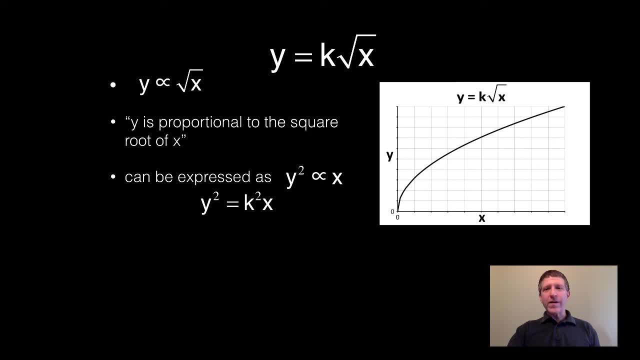 Squaring both sides, you get y squared equals k squared times x. That's going to come in handy later, as we much prefer squaring numbers than taking the square root. You're going to see, we're going to need to do this. We're going to transform a square root relationship by squaring both sides into a square relationship. 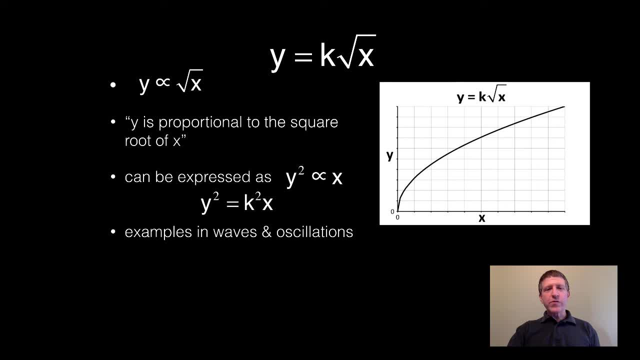 Makes things somewhat easier. There's a bunch of examples. There's a few from waves and oscillations of this type of relationship, And we have the period of the pendulum equaling 2 pi times the square root of l over g. That is a relationship that we're going to take a much closer look at in the next video. 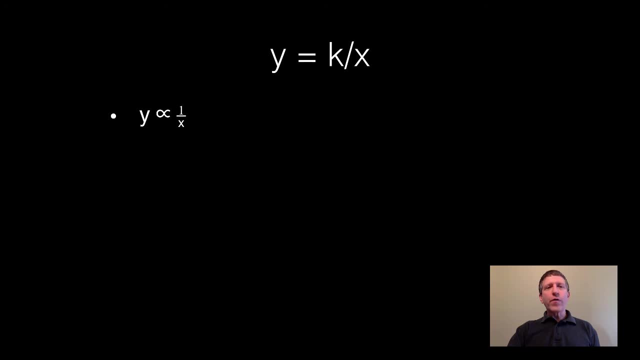 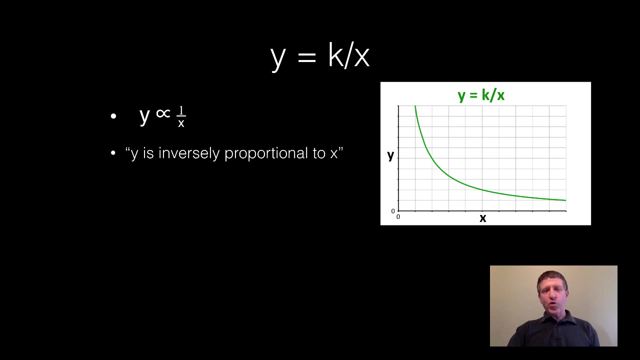 This relationship is also very common: y equals k over x. When you say this, you simply say y is inversely proportional to x, which means the same thing as y is proportional to 1 over x. It is just as common as direct. 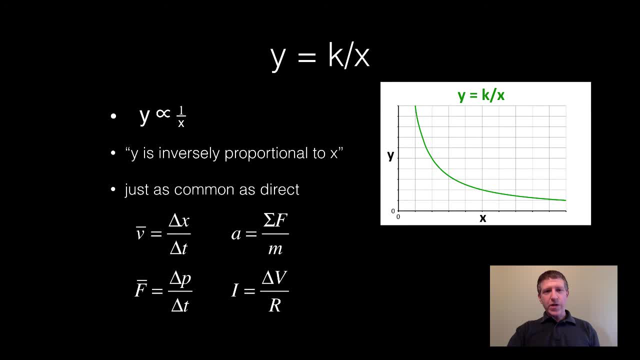 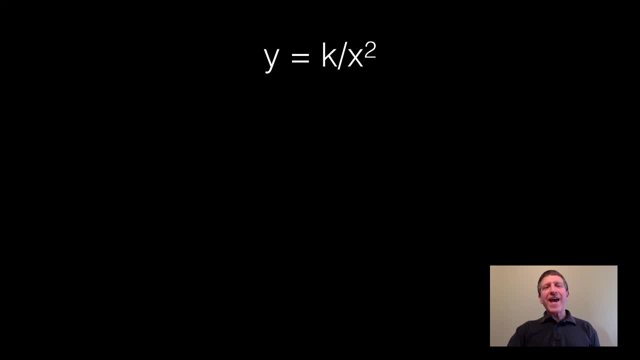 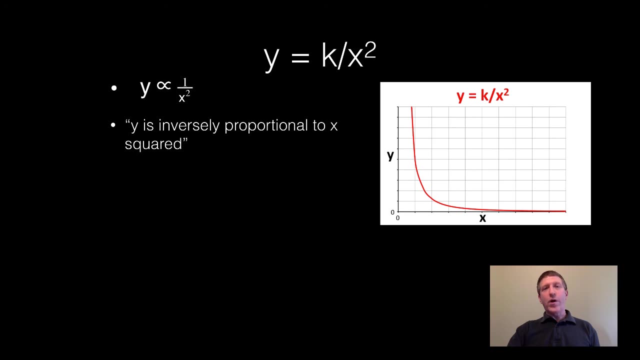 And you can write many direct relationships as an inverse relationship. Here are some examples. Another common relationship: y equals k over x squared. You can say y is inversely proportional to x squared. or you could say y is directly proportional to 1 over x squared. 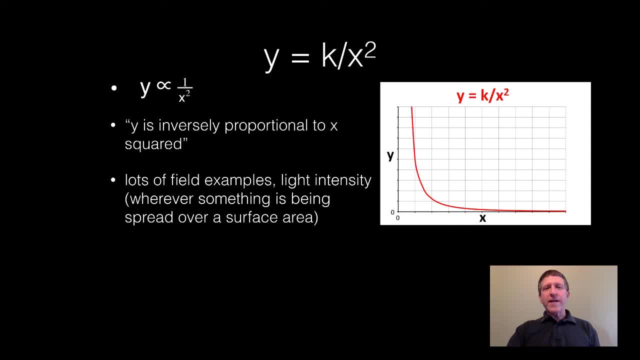 There are a lot of examples in this, especially in fields and light intensity: Whenever you have something that's being spread out over a surface area, like light that's spread out over a sphere, for example, In fact, with stuff like gravity. 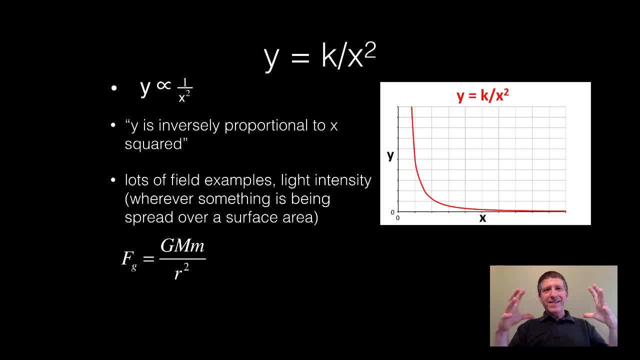 we have what's called gravitational flux lines are spread out over a sphere. So that's one way of looking at why the force of gravity is gmm over r squared. It's being spread out over an area. We also have electric fields And light intensity, as I mentioned before.